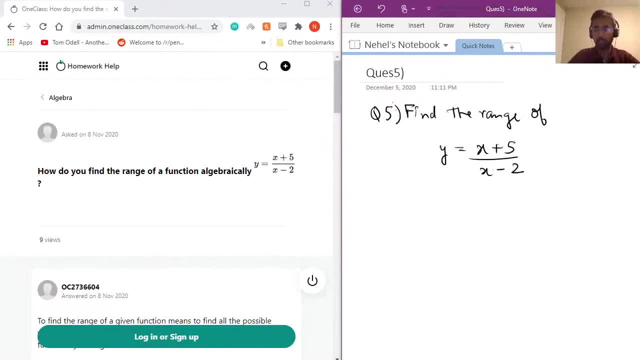 over x minus two. So, first of all, what is the range? So the range of a function is all the values of the function Can take without it being non-real or non-solvable. In this case, the range of this function would: 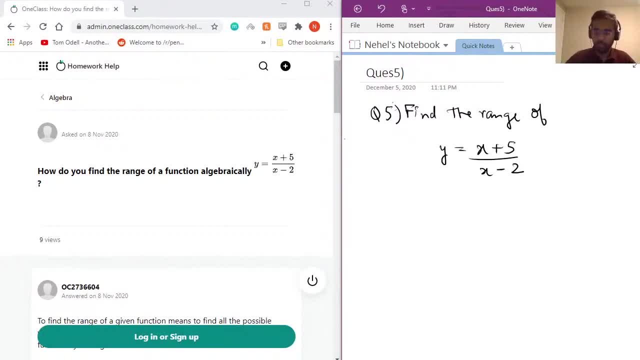 be all the possible values of y. So we're trying to find, trying to find all possible values that y can take, Okay. Similarly, even though this question does not ask for it, we'll just briefly touch upon it. If we were to ask for the domain, the domain would: 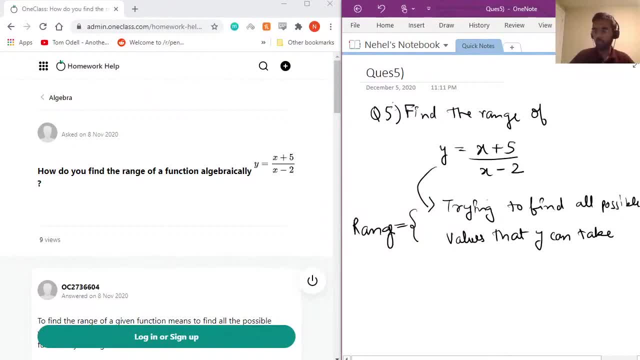 be all possible values which x can take. So in this case we're not being asked for it, but that's how we define the domain. In this case, the way we would be able to find out um all possible values for y is 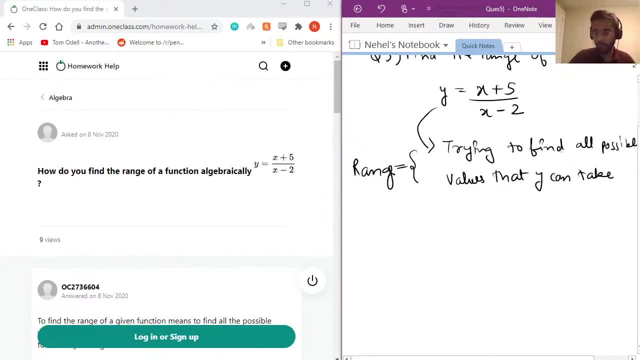 you would have to solve for x. So I'll show you. I would do that in just a second. but let's first solve for x. So the way we would do that is we would cross multiply. the denominator with the left-hand side is equals to x plus five. So y, x minus two, y is equals to x plus. 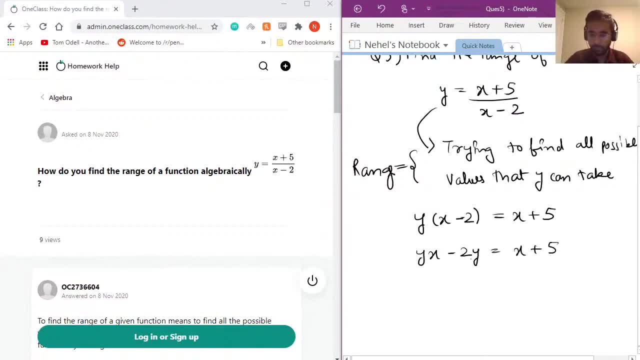 five. This goes to the other side. x becomes common x minus sorry, x of y minus one minus two y. Okay, So now this is the same thing that you would do for y, So you would take x to the left. 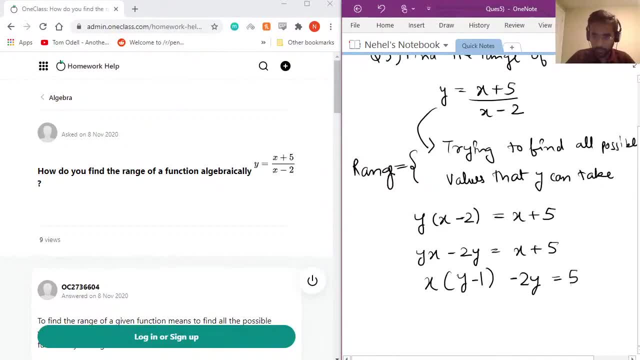 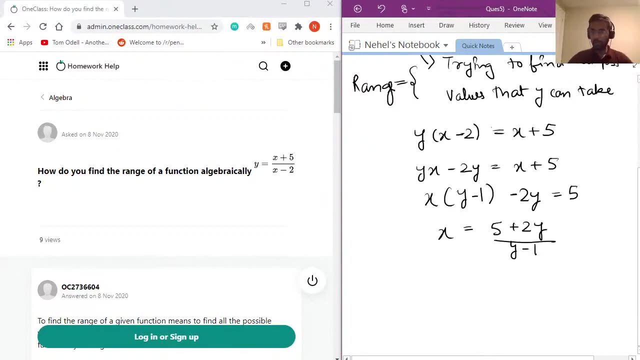 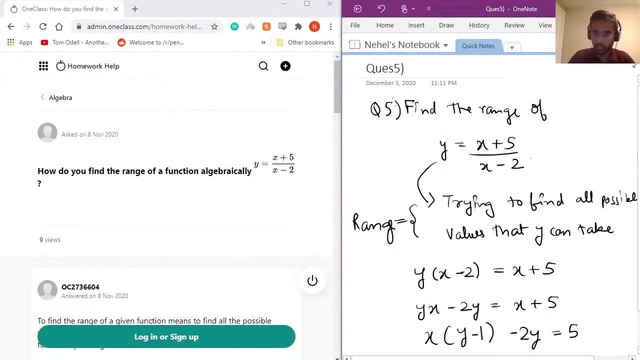 So you would take: x to the right is equals to 5, x is equals to 5 plus 2y over y minus 1. okay, so the way we solve for y is: first we took the numerator or the denominator of the initial equation, so we took this: 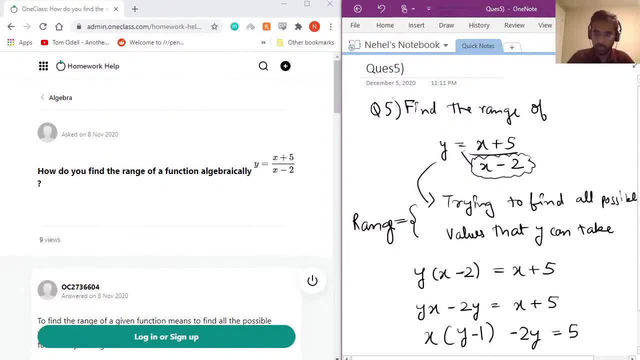 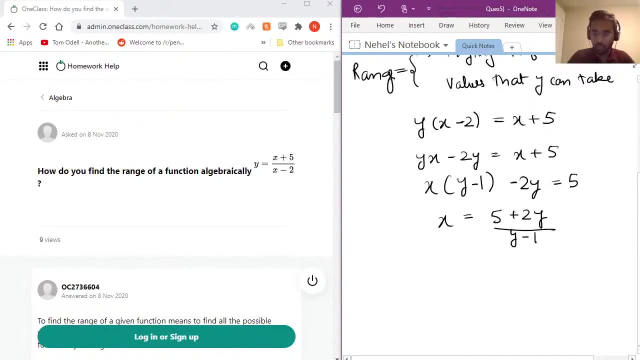 and we cross multiplied it to the other side. after that we opened the bracket and we solved for the final expression. after solving for that, we took the x to the other side, and when we took negative 2 to the other side- once we took the x to the other side- we actually saw that we have 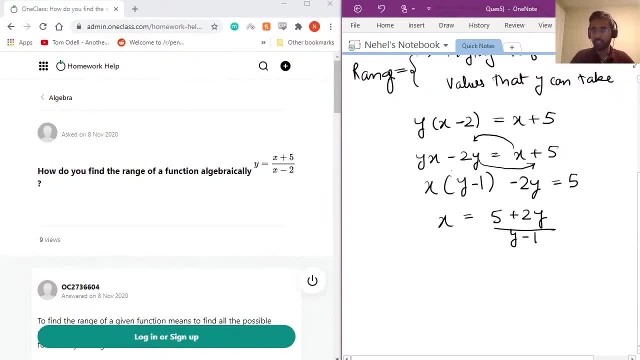 term y, x and negative x on the same side, so we can extract x to be the common term from 2 and we are left with x times y minus 1. after that, the final step was to send y minus 1 back to the denominator on the right hand side. okay, so now that we have solved for y or y in terms of x, 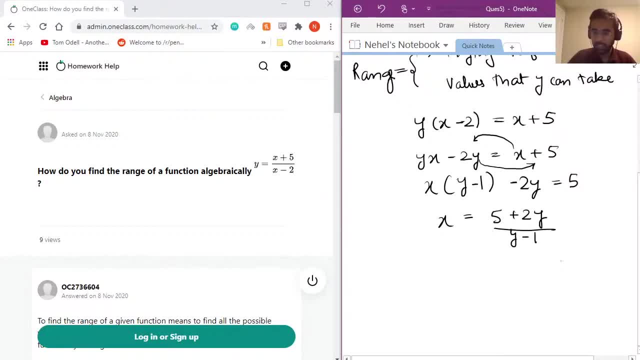 we can say that just by looking at this, we know that x is defined for all values of y, but for y equal to 1, because when y equals to 1, this terms becomes 0 and any number but divided by 0 is in defined. so that would be a problem. so we can say that I cannot be equal to 1. okay, and that is. 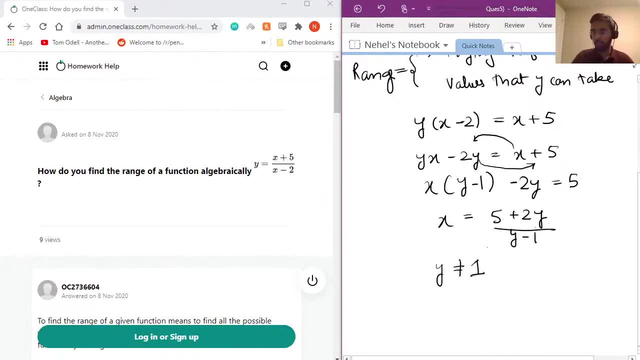 the only way to solve the problem. number which would pose a problem. all of the numbers are part of the range, whereas y, equal to 1, is not part of the range. okay, therefore, the range of the function y is equals to x plus 5 over x minus 2 is? you have to be a bit careful? 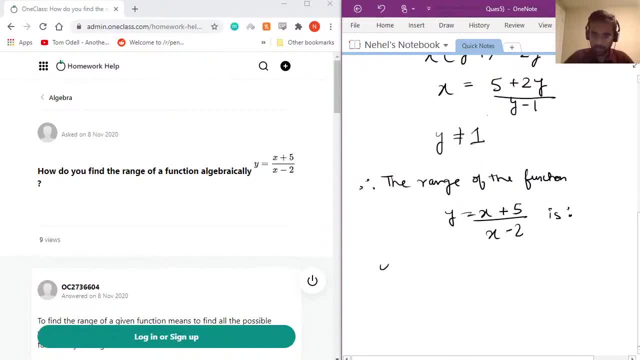 with the notation here. so the way we express range is: y belongs to a subset. the subset would be from negative infinity to the negative infinity and the subset would be from negative infinity to the negative infinity and the subset would be from negative infinity and the subset would be from negative infinity and the subset.